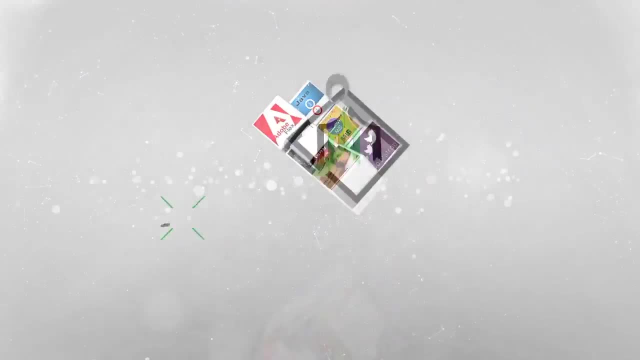 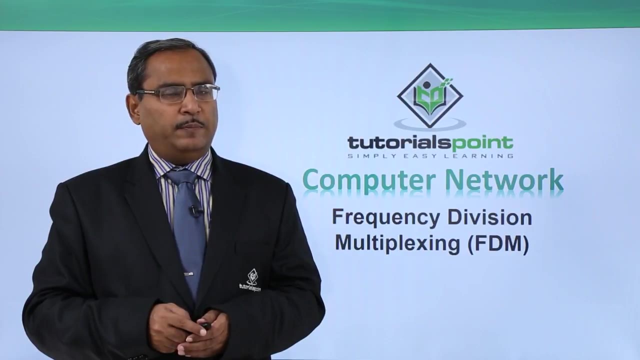 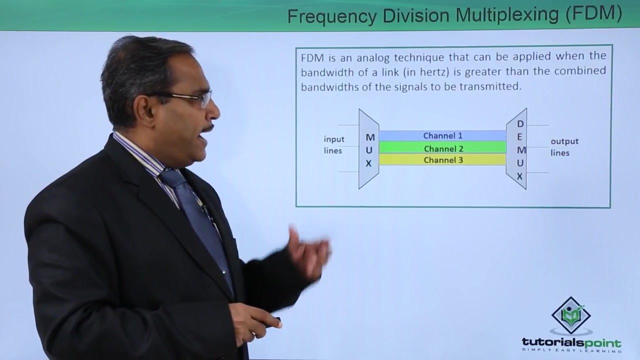 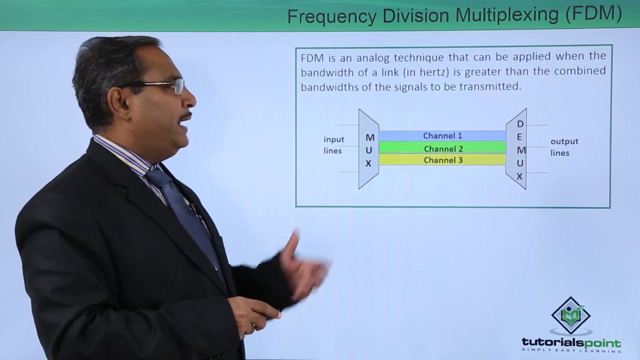 In this video we are discussing frequency division multiplexing. in short it will be called as FDM. So FDM is an analog technique that can be applied when the bandwidth of a link in hertz is greater than the combined bandwidths of all the signals which are to 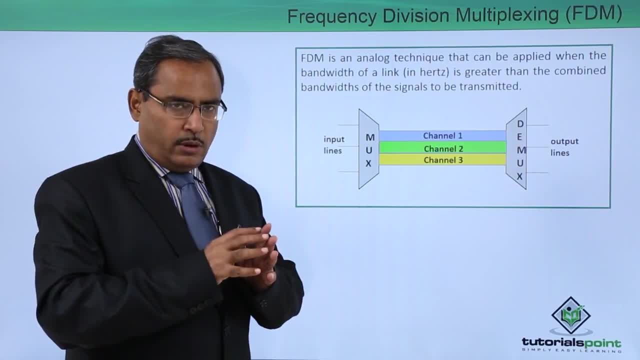 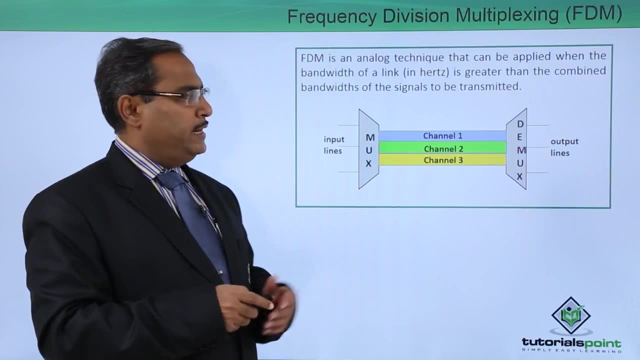 be transmitted When the signal bandwidth, combining all the signals which are to be transmitted, if it is greater than the bandwidth allowed in the respective medium, in the respective link. So in that case we will be going for this frequency division, multiplexing Then. 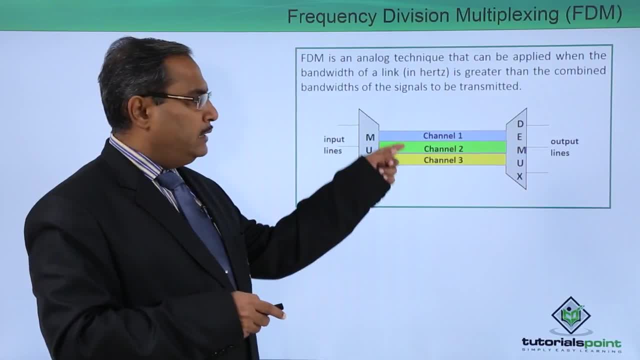 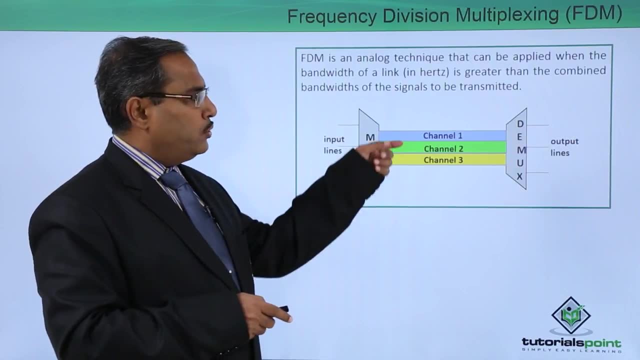 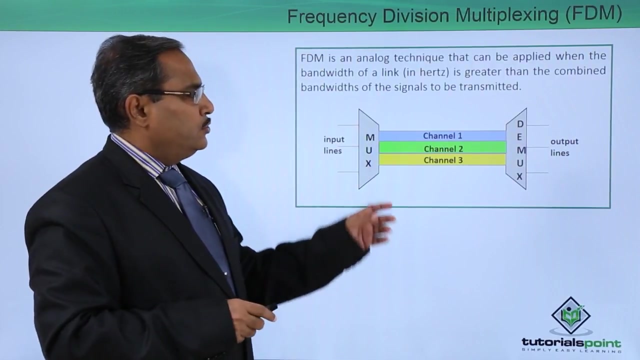 what will happen? we will be dividing this particular link into multiple channels, and all this particular channels are having some inter separation gap, So also known as inter channel gap. So this is the forbidden gap, so that the channels should not get mix up. So these 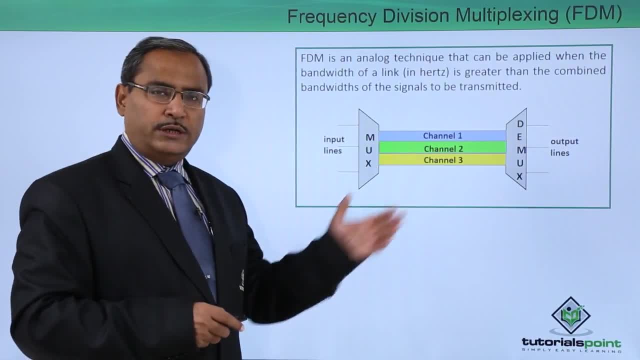 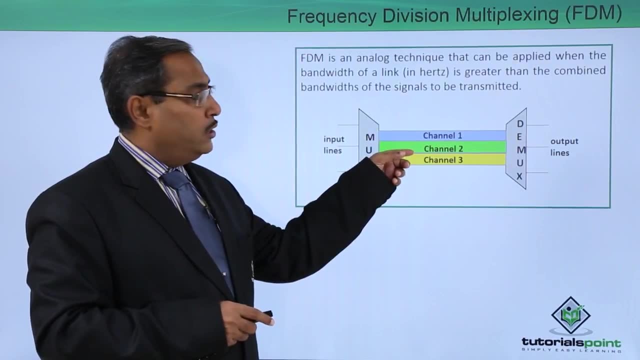 are, the gaps will be there. So how many channels are there? we have shown here 3.. So how many such guard bands will be required? forbidden channel, forbidden gaps are required. So here we will be requiring two of them. So here we are having this. input lines: the respective. 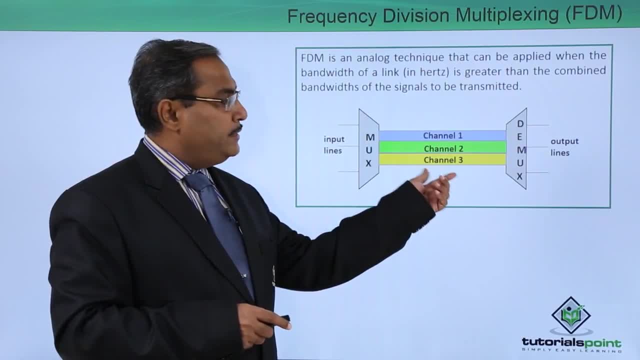 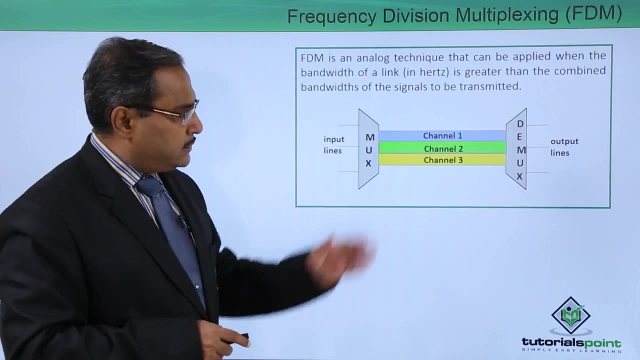 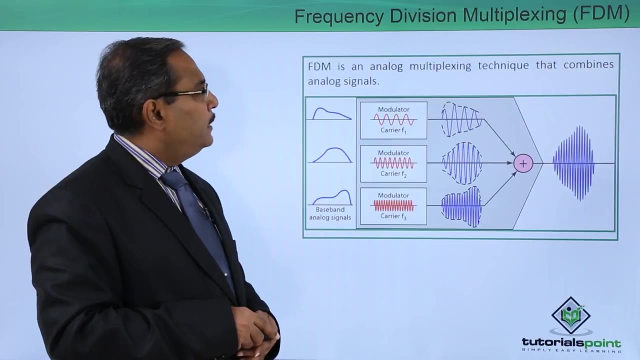 multiplexer. we are having channels are getting created or defined, and then, through each and every channel, the data is getting transmitted. At the receiving end, we are having the DMUX and the output lines will be obtained accordingly. So let us go for another diagram for the better understanding. So FDM is an analog. 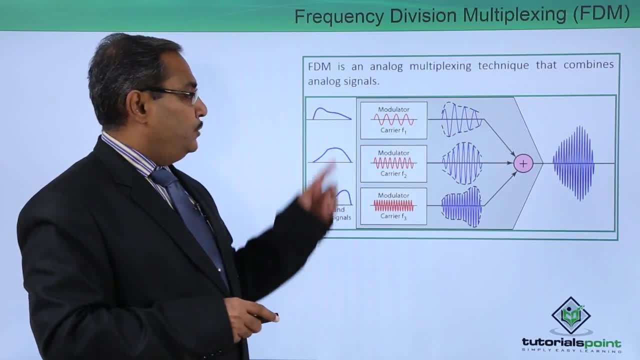 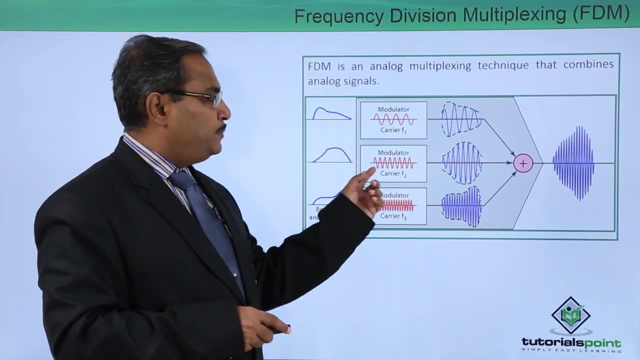 multiplexing technique that combines analog signals. So here you see, here we are having multiple analog signals are there. So baseband analog signals are there, and these are the respective modulators having got different carrier frequencies, let it be F 1,, F 2 and 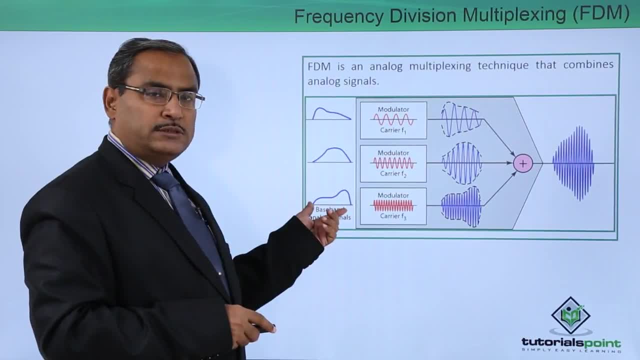 F 3, you can get it from here. So this particular signal is getting transmitted. So this particular signal is getting transmitted. So this particular signal is getting transmitted. So this particular analog signal will be modulated with using this carrier frequency. So here also, and 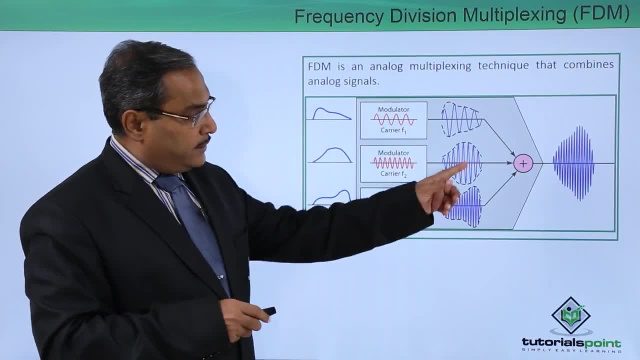 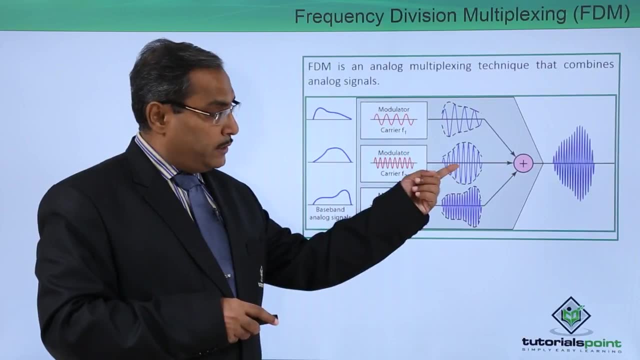 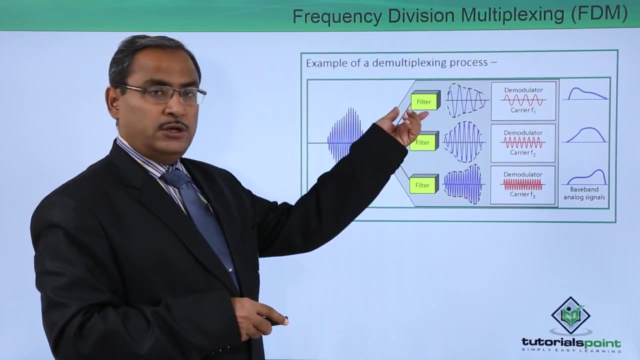 here also. now I shall go for addition and then the resultant, the resultant analog signal which will be transmitted through the media, will be: look, will be looking like that, And then at the receiving end, we will be having the respective filters, so that I can get. 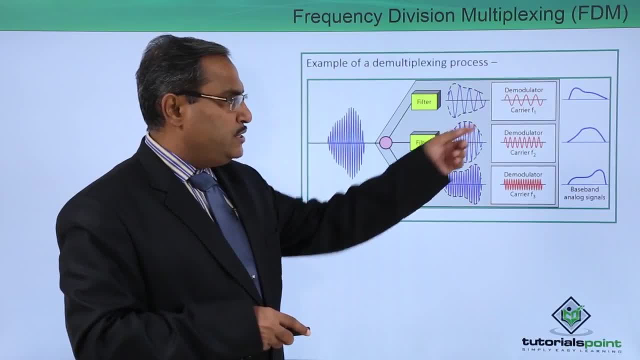 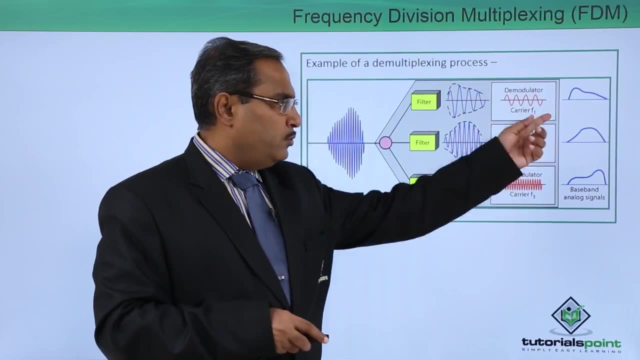 back my channel data accordingly, and then we are having this demodulator will be which will be working with this frequency for this one, with this frequency for this one行 this frequency, Then we will be getting our baseband analog signals at outcome. 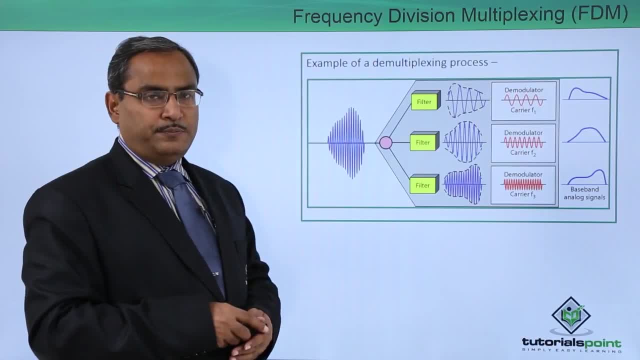 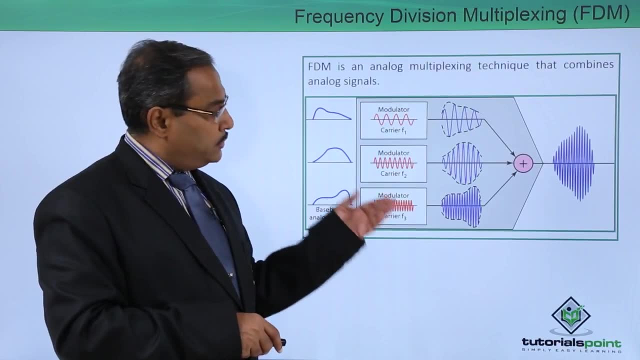 So, in this way, the examples of demultiplexing process we have discussed in the previous slide, we discussed the the example of multiplexing processes. So this is about multiplexes where it will be done at the central part, and this is about demultiplexing process. 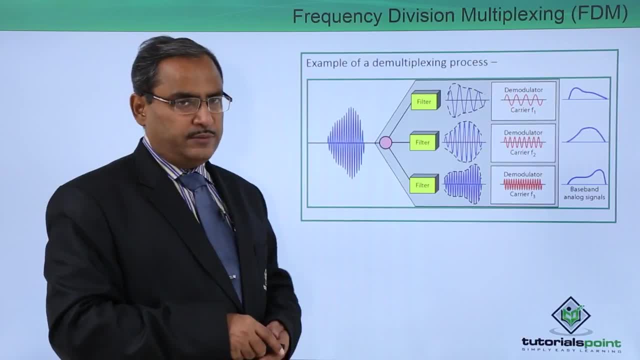 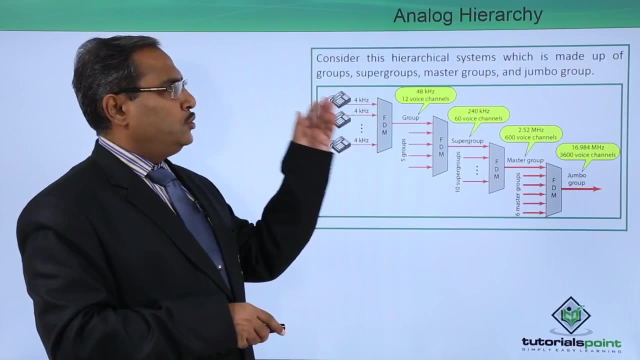 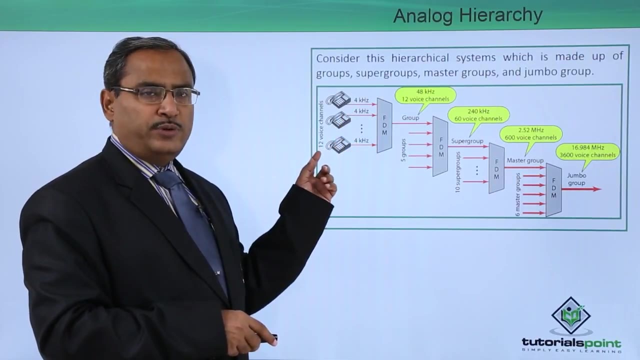 where it will be done at the receiving end, at the receiving end. So consider this hierarchical system, which is made up of groups, super groups, master groups and jumbo group. So how many voice channels were having? there is a 12 voice channels. So this FDM will form it in a group, a single group. how many groups are there in? 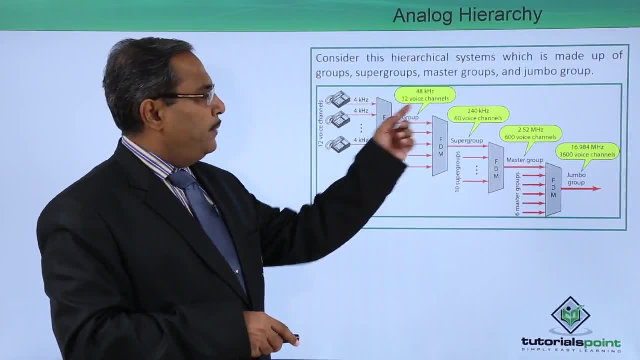 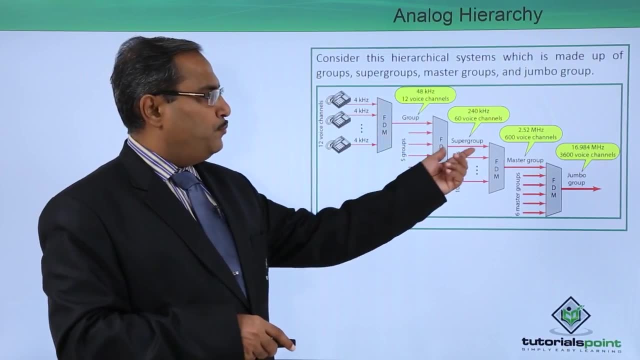 total. in this way we are having 5 groups. So here we are having 12 voice channels for each and every group, but 5 groups such will be there. So this FDM will produce a super group which will be having 60 voice channels. So how many such super groups are there? 10.. 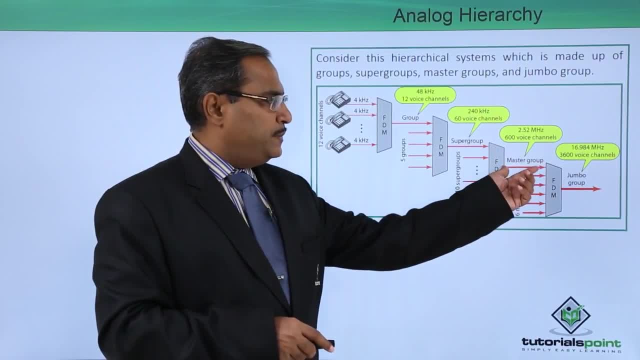 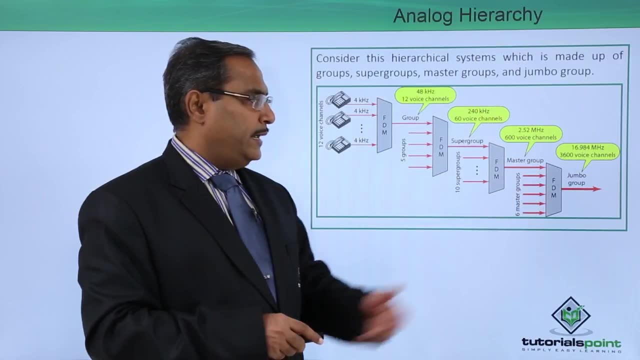 So 16 to 10. how many voice channels are we expecting in the master group? So we are having 600 master groups were having 600 voice channels were having in each and every master group. how many such master groups are there? 6 master groups. So that is our jumbo group. 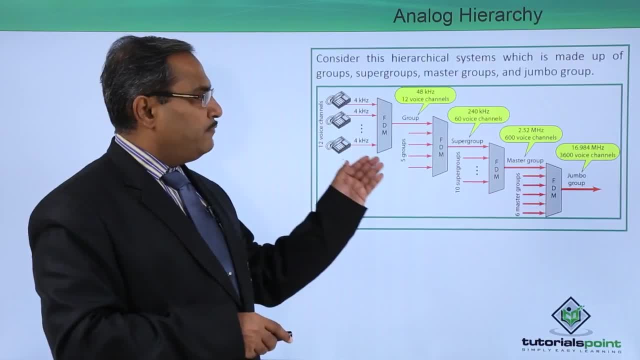 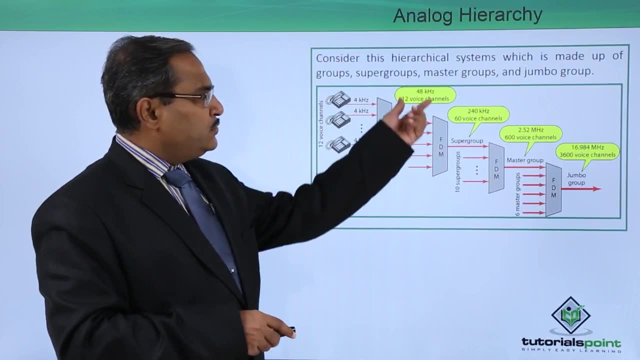 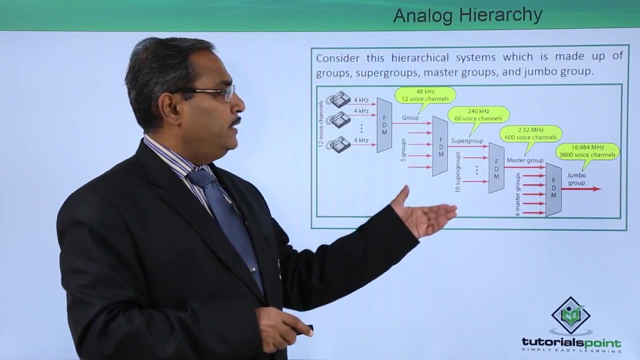 of 3600 voice channels. So in this way you can find that we are having the conception of group, super group, master group and jumbo group and in this way, if you go on calculating the respective frequencies, you will be getting the answers in this way. So this is our analog hierarchy, where we 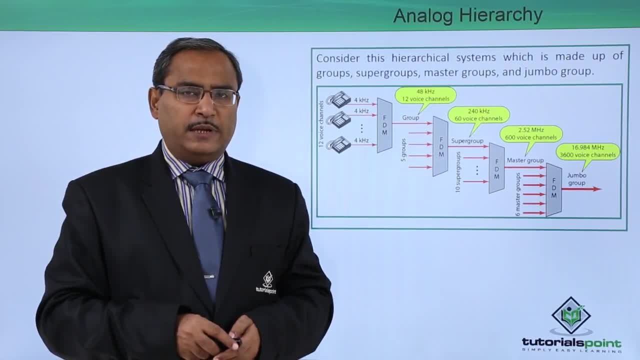 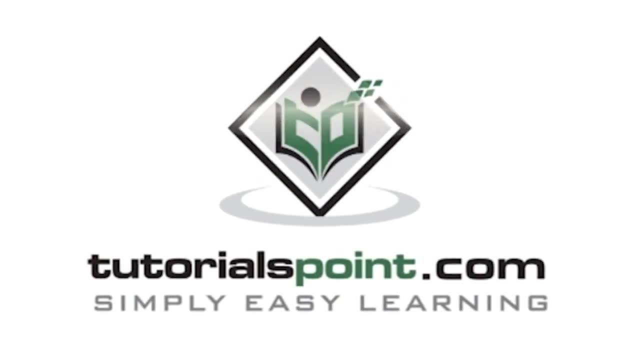 are showing you that how this frequency division multiplexing is working here. Thanks for watching this video.